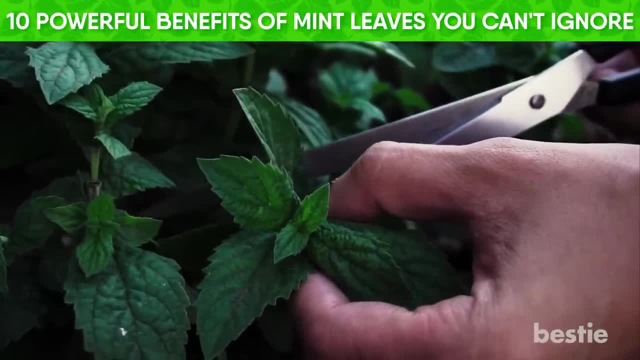 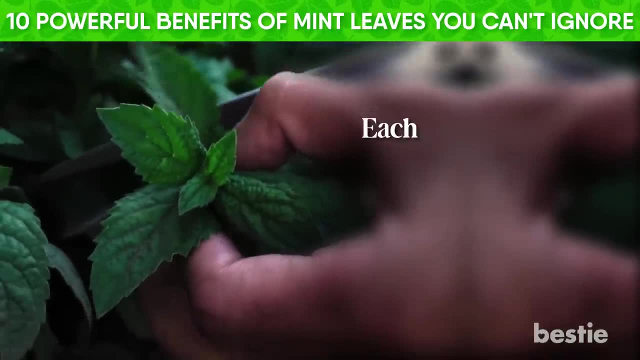 Since ancient times, people have used various types of mint all over the world. There are varieties of mint plants that offer a lot of antioxidant properties and health remedies. Each is packed with phytonutrients containing vitamin C, A, B-complex, phosphorus, calcium. 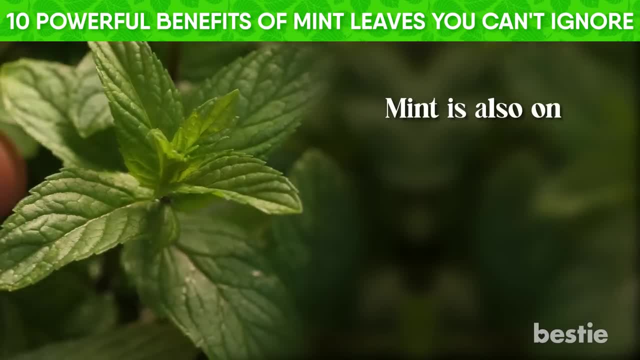 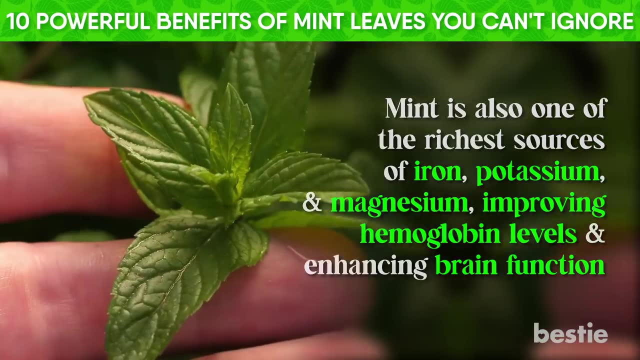 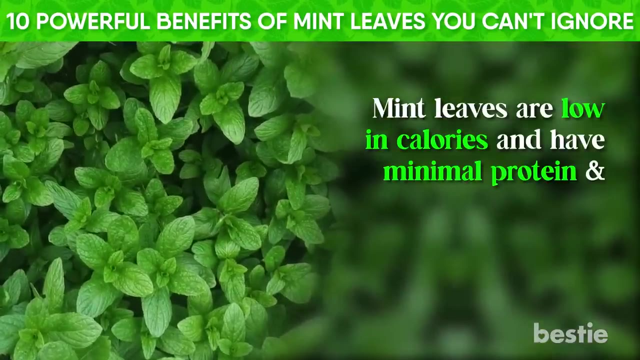 and antibacterial properties. Mint is also one of the richest sources of iron, potassium and magnesium, improving hemoglobin levels and enhancing brain function. Think that's all Not quite. Mint leaves are low in calories and have minimal protein and fat, so you can easily add mint leaves to your weight loss diet. Isn't that great? 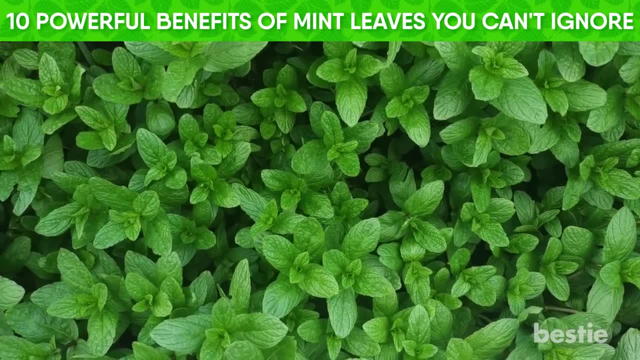 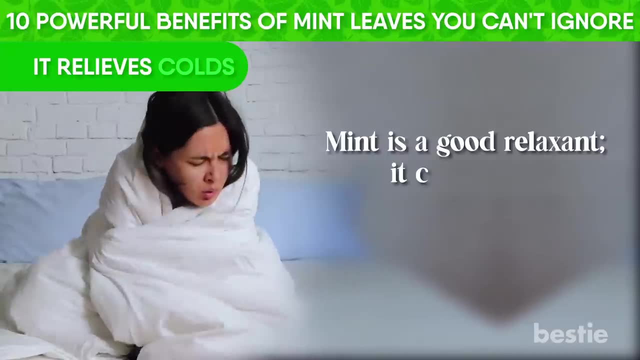 Now let's get right into the health benefits of mint. It relieves colds. Mint is a good relaxant. It can help relieve throat nausea and fever. Mint is also a good relaxant. It can help relieve throat nausea and fever. Mint is a good relaxant. It can help relieve throat. 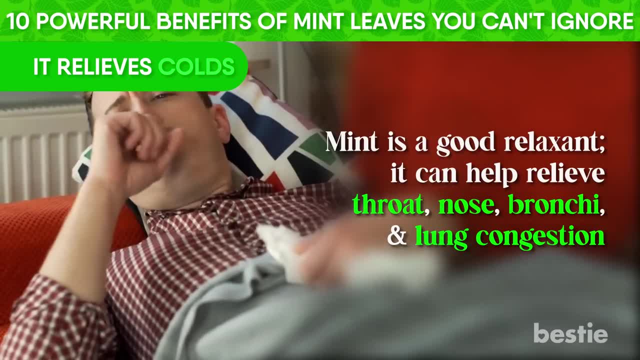 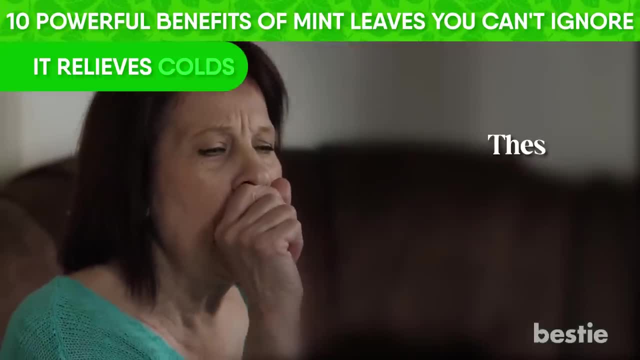 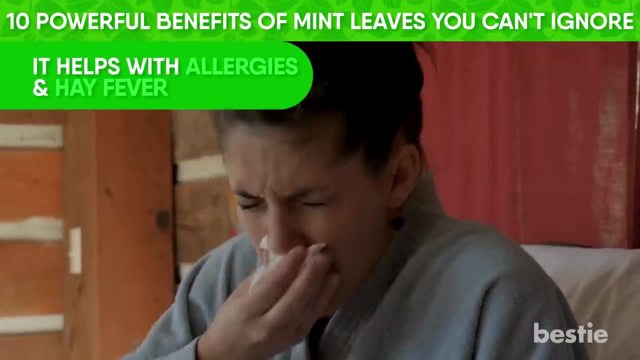 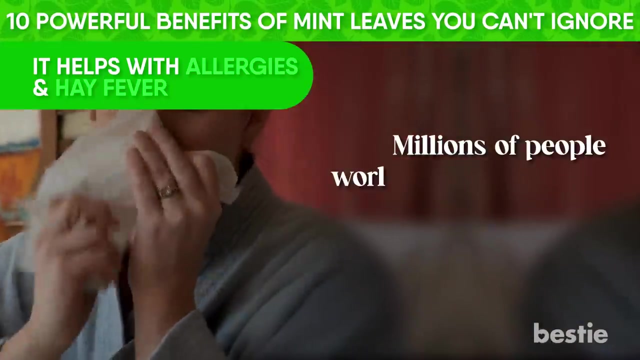 nose, bronchial and lung congestion. Its anti-inflammatory properties also help reduce the irritation caused by chronic coughing in respiratory channels. These are prime reasons why your vapor rubs and inhalers contain mint. It helps with allergies and hay fever. Do you ever get seasonal allergies? You're not the only one: Millions of people worldwide. 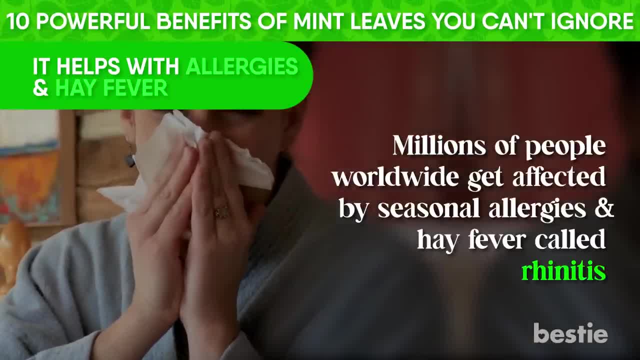 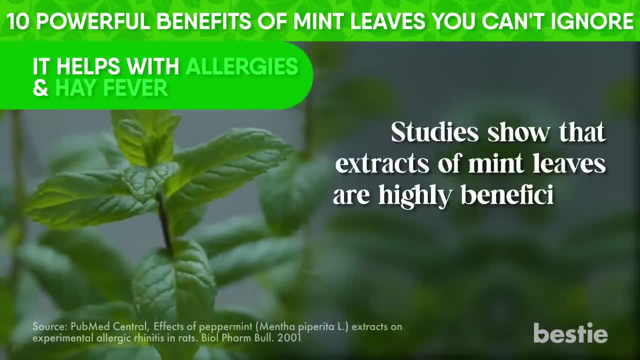 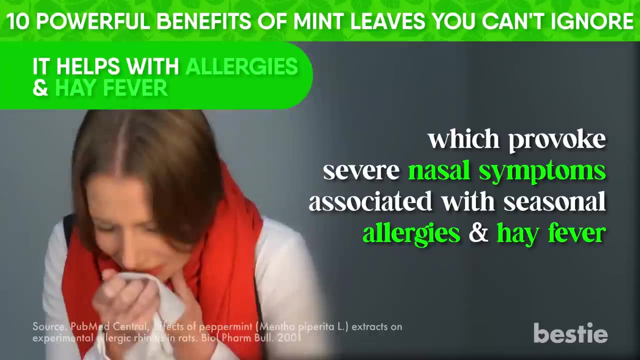 are affected by seasonal allergies and hay fever called rhinitis, But mint leaves are a great solution to your seasonal sniffles. Studies show that extracts of mint leaves are highly beneficial in preventing the release of certain chemicals which provoke severe nasal symptoms associated with seasonal allergies and hay fever. 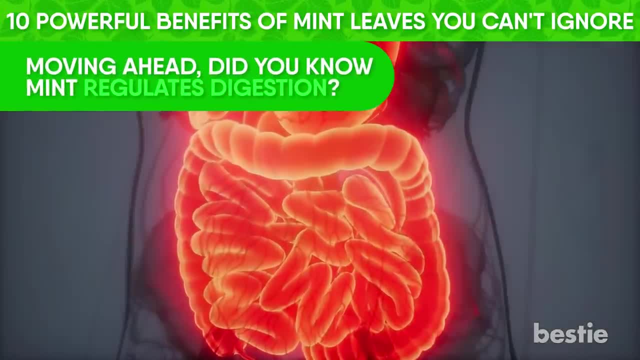 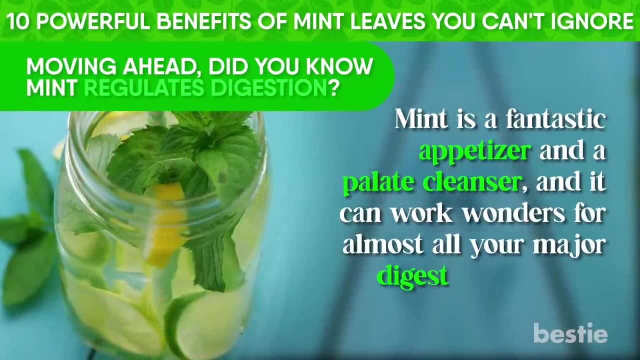 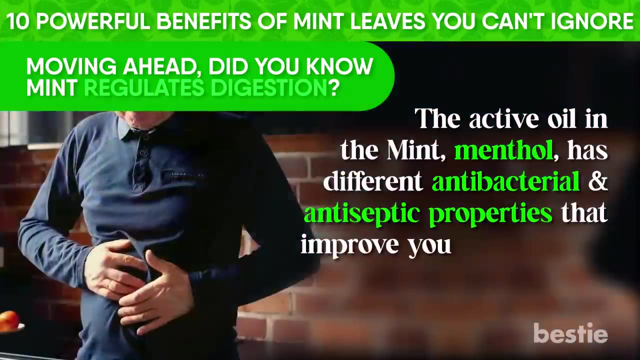 Moving ahead. did you know? mint regulates digestion? Mint is a fantastic appetizer and a palate cleanser. It can work wonders for almost all your major digestive problems. The active oil in the mint, menthol, has different antibacterial and antiseptic properties that improve your digestion and settle an upset stomach. 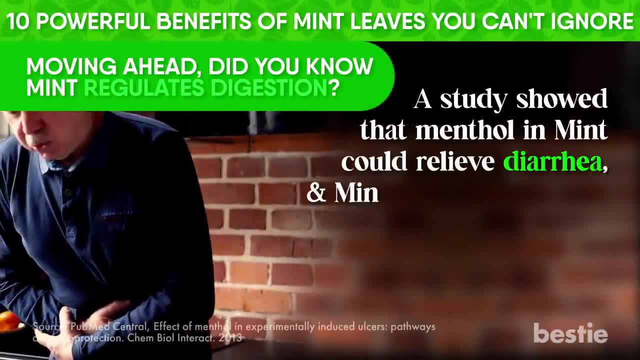 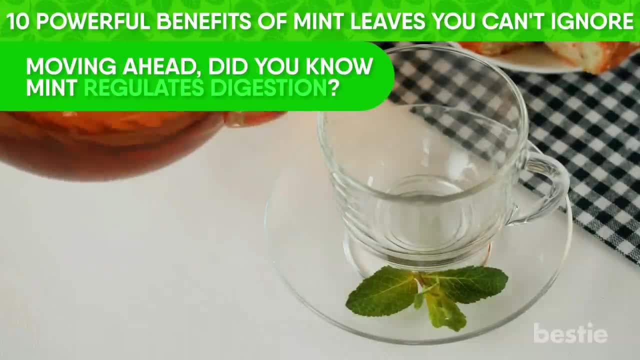 A study showed that menthol in mint could relieve diarrhea, and mint is also a powerful remedy for relieving irritable bowel syndrome symptoms. So the next time you're not feeling too good down there, make a nice cup of mint tea to help relieve your digestive system. 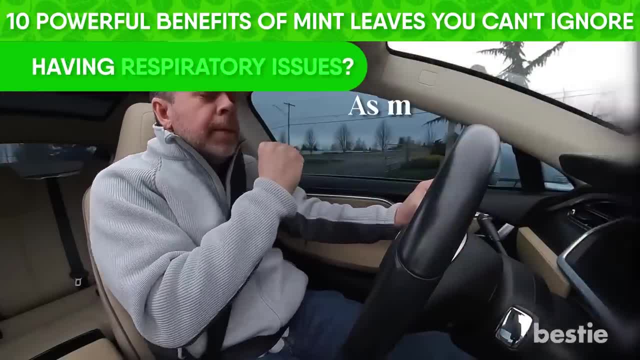 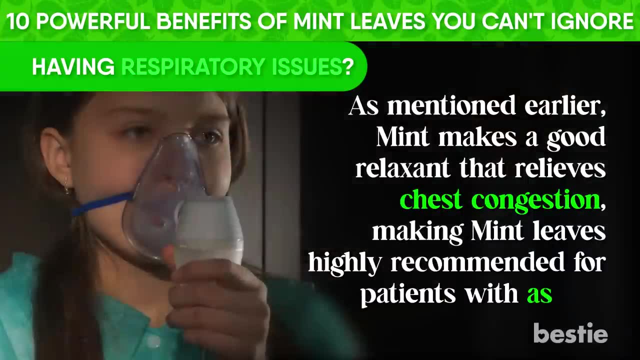 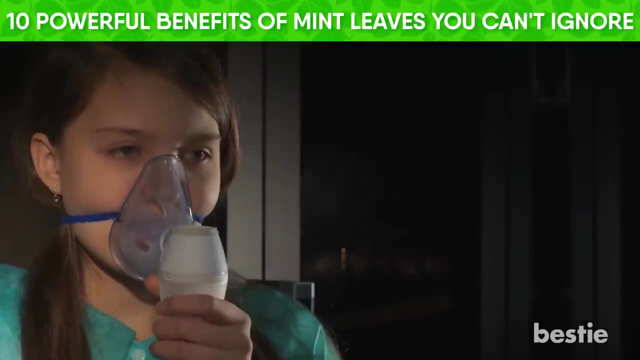 Having Respiratory Issues. As mentioned earlier, mint makes a good relaxant that relieves chest congestion. Making mint leaves is highly recommended for patients with asthma. Consuming mint can be very relaxing for asthmatic patients and others with respiratory disorders, Not to mention how great it is for your skin. 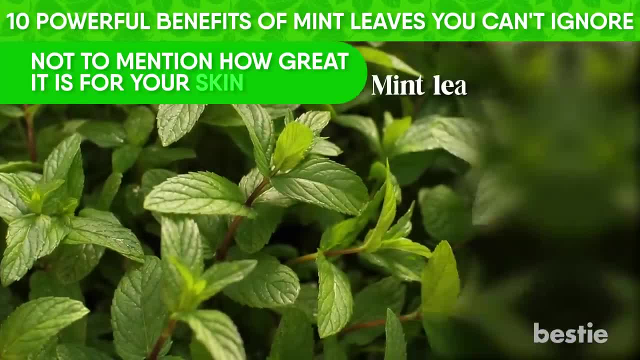 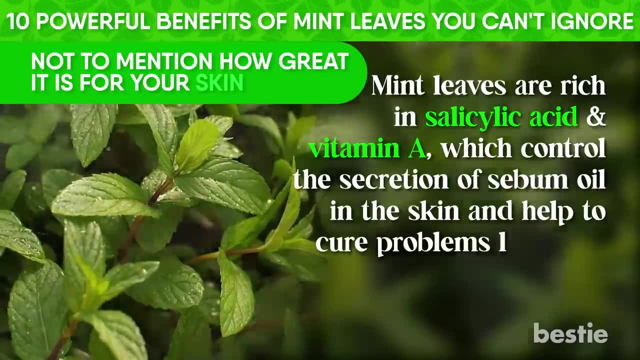 Mint has been used for centuries to treat skin problems. Mint leaves are rich in salicylic acid and vitamin A, which control the secretion of sebum oil in the skin and help to cure problems like acne and redness associated with acne outbursts. It's great for toning. 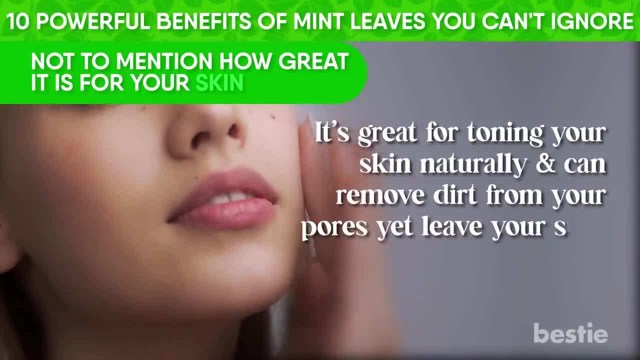 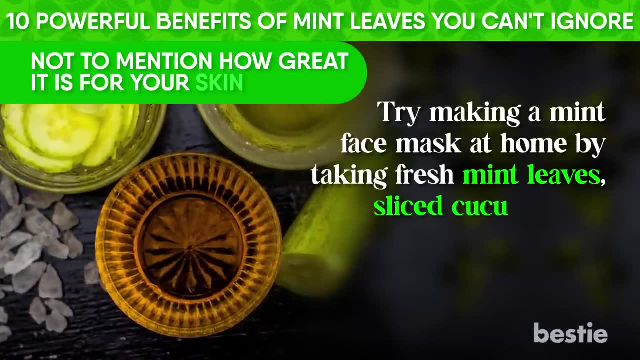 toning your skin naturally and can remove dirt from your pores yet leave your skin feeling smooth and hydrated. Try making a mint face mask at home by taking fresh mint leaves, sliced cucumber and honey and blending it into a smooth paste. Apply to your face, then rinse with cold water after. 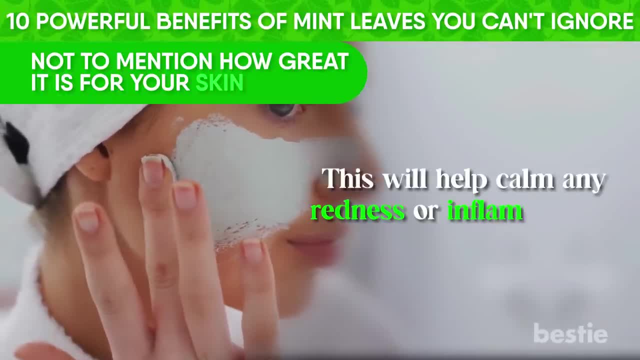 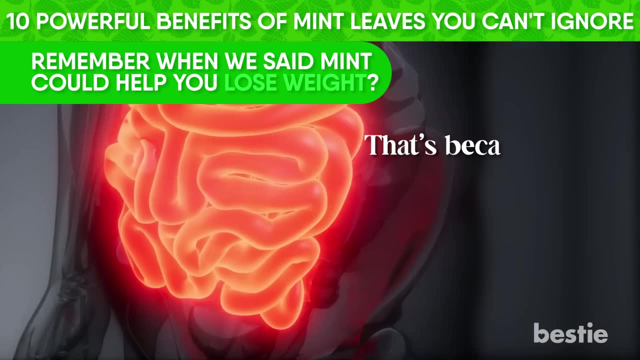 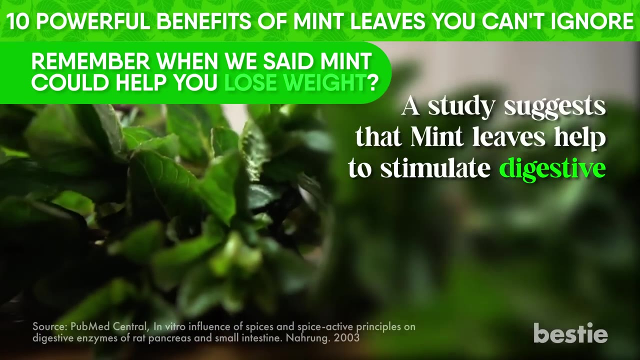 15 minutes. This will help calm any redness or inflammation. Remember when we said mint could help you lose weight. That's because mint leaves enhance digestion and boost your metabolism. A study suggests that mint leaves help to stimulate digestive enzymes, which absorb. 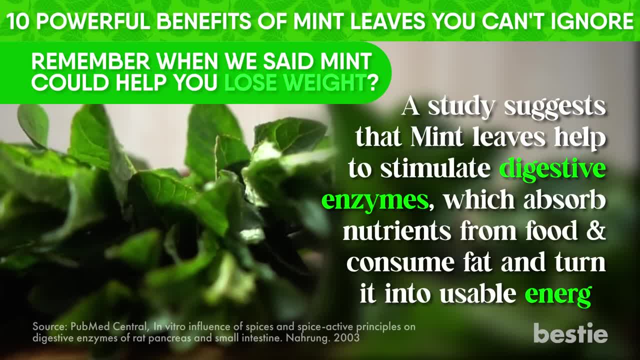 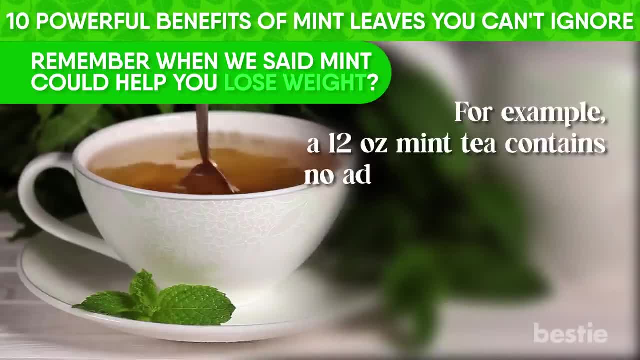 nutrients from food and consume fat and turn it into usable energy. Also, having mint tea can benefit due to its low calorie count. For example, a 12-ounce mint tea contains no added sugar and has no calories, while a 12-ounce soda has 37 grams of sugar and. 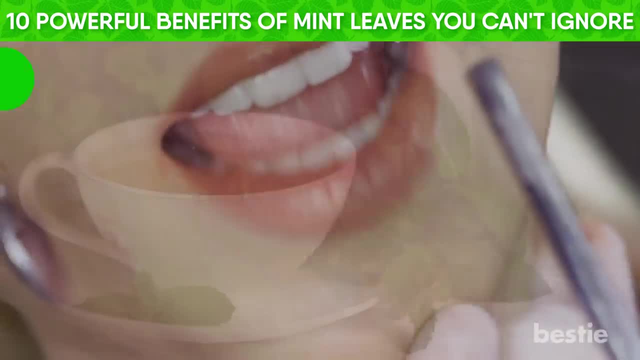 150 calories. Mint takes care of your oral care. Next time you need to eliminate a strong smell from your breath, you can take a sip of mint. The mint leaves are rich in vitamin A, vitamin C and vitamin C. Mint leaves are rich in vitamin. 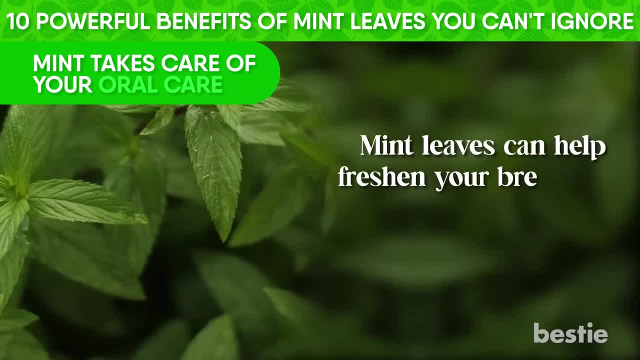 X and vitamin D, which help you to lose weight. If you have a weak palate or can't breathe properly, try eating mint leaves. Mint leaves can help freshen your breath in no time due to their germicidal properties. That's why. 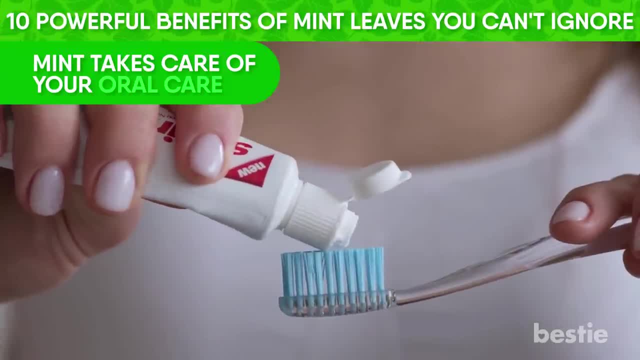 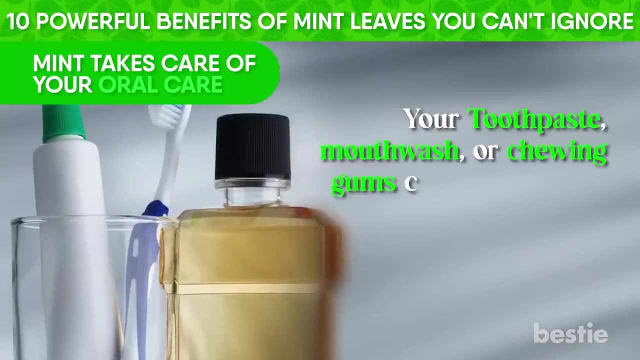 it's in almost all oral care products, such as toothpaste and gum. Mint leave extract can also help to clear plaque. Your toothpaste, mouthwash or chewing gums contain menthol, which removes oral bacterial growth and keeps your oral cavity clean. 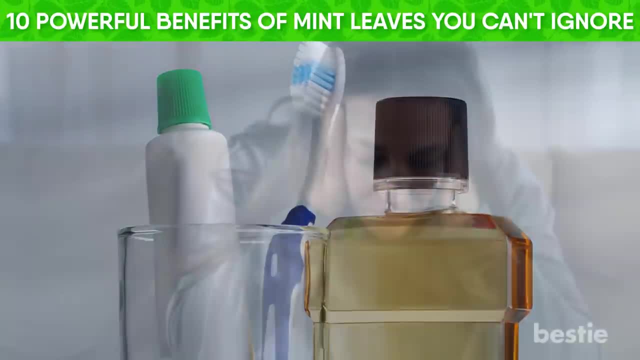 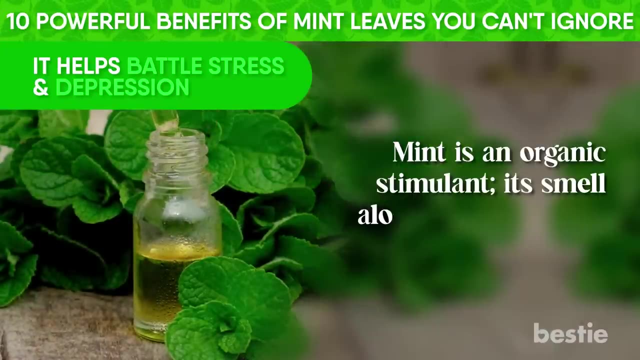 Mint doesn't just keep your oral hygiene healthy. it helps battle stress and depression. Mint will help further reduce the risk of oral activity by retaining it for a long time. Mint does. Mint is an organic stimulant. Its smell alone can be enough to uplift your mood. 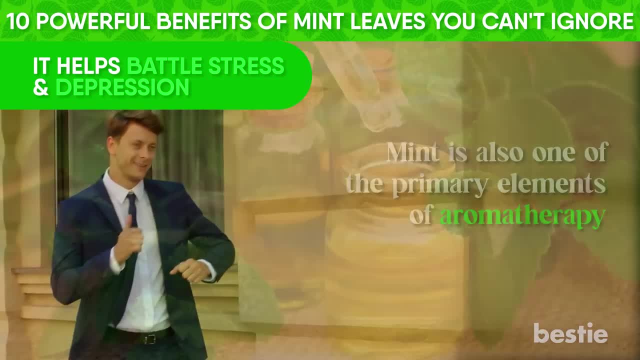 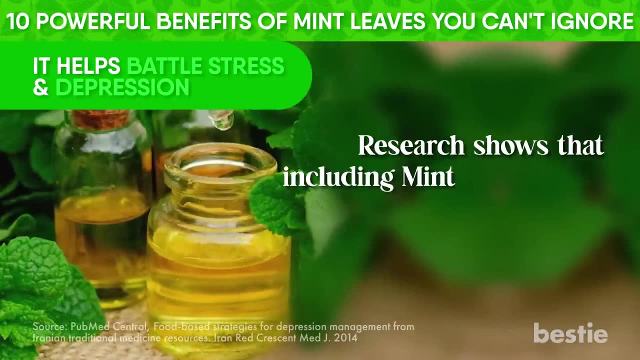 Mint is also one of the primary elements of aromatherapy. Its refreshing and robust fragrance can help you battle stress and refresh your mind. Research shows that including mint in your diet can be fantastic, because the herbal leaves and their essential oils can help if you feel anxious. 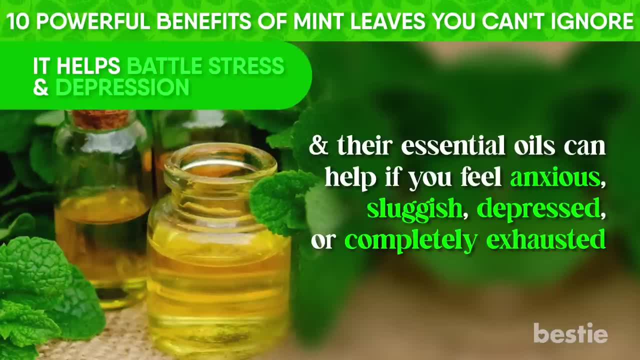 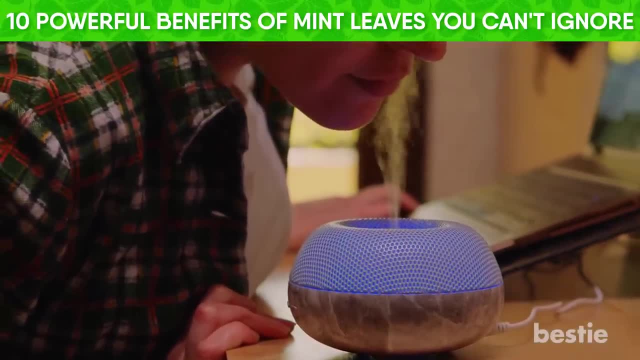 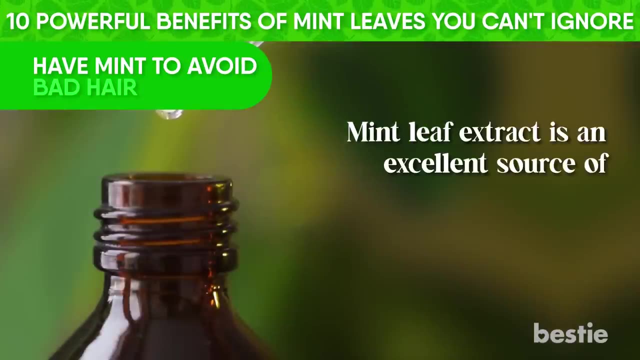 sluggish, depressed or completely exhausted. Use mint extracts on a vaporizer or take a bath with mint for instant relief from stress and depression. Have mint to avoid bad hair. Mint leaf extract is an excellent source of carotene and antioxidants that promotes hair. 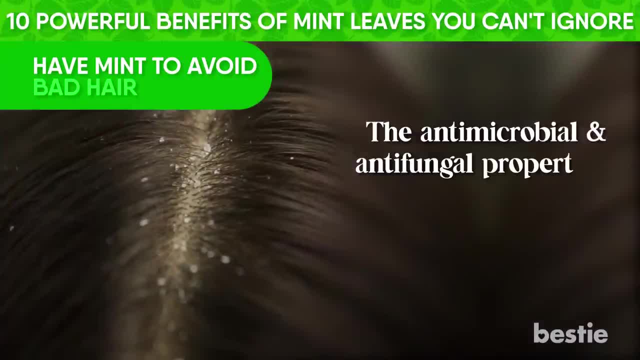 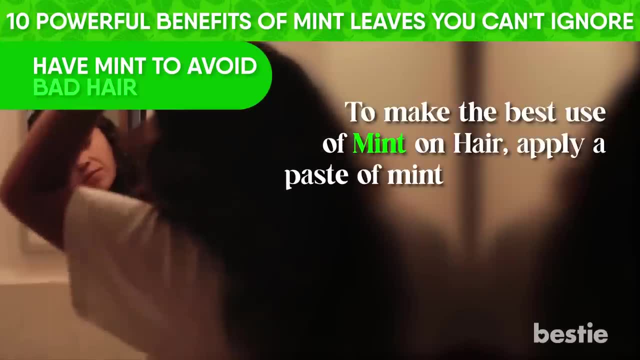 growth and reduces hair fall. The antimicrobial and antifungal properties of mint leaves can also be used to ward off dandruff. To make the best use of mint on hair, apply a paste of mint leaves mixed with lemon juice on the scalp. 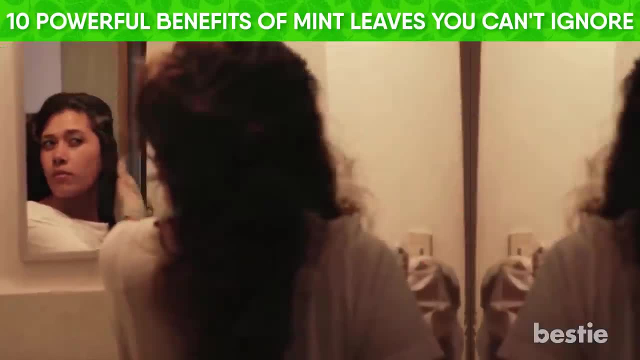 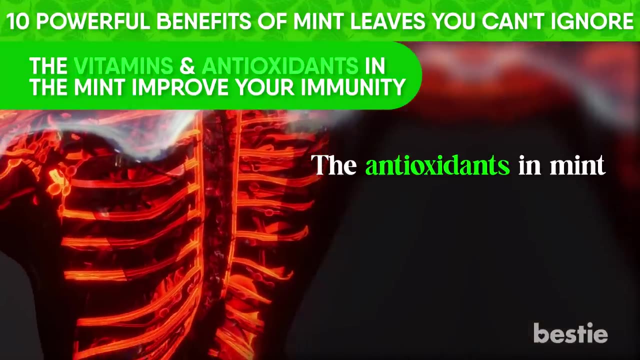 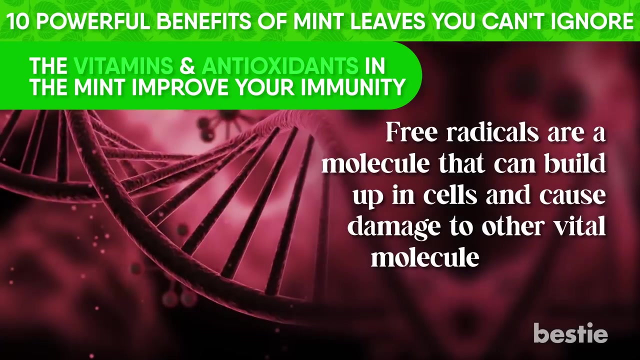 Let it stay for 30 to 40 minutes and rinse well. The vitamins and antioxidants in the mint improve your immunity. The antioxidants in mint help prevent free radical activity in your body. Free radicals are a molecule that can build up in cells and cause damage to other vital molecules. 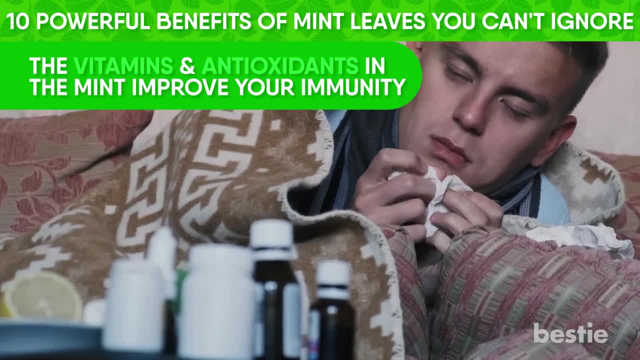 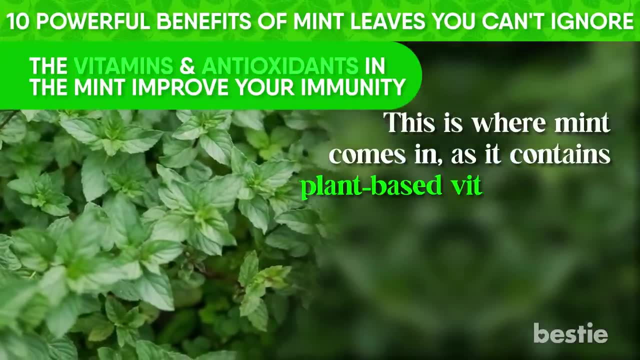 like DNA or protein, Because free radicals are unstable. they can cause illness and aging, which is something the body tries to prevent. This is where mint comes in, as it contains plant-based vitamins that can help to protect yourself and prevent hair loss. Mint is also a good source of vitamin C and vitamin E. 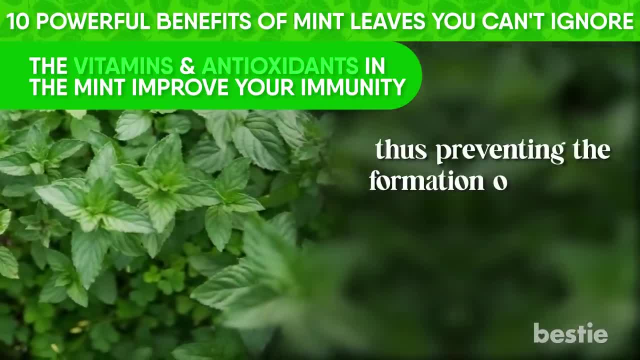 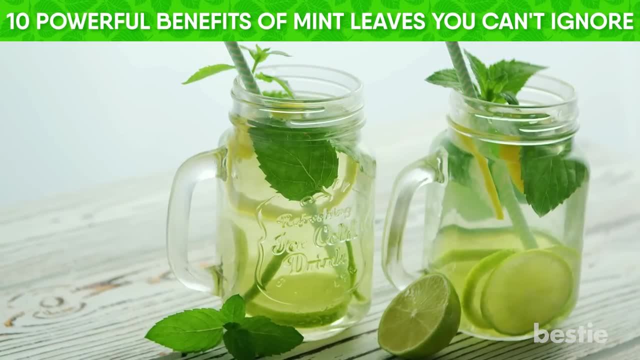 It is also a mineral for the body which is responsible for a healthy body. Mint leaves help you recover cells from the damage caused by free radicals, thus preventing the formation of various tumors by inhibiting some enzymes. Add mint to your diet. Adding mint to your diet is easy. Mint leaves make for a perfect garnish to your cocktails. 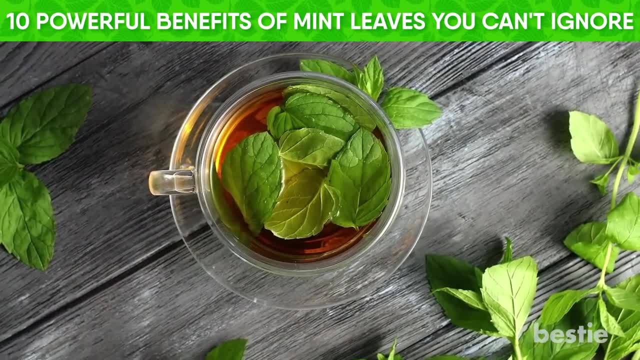 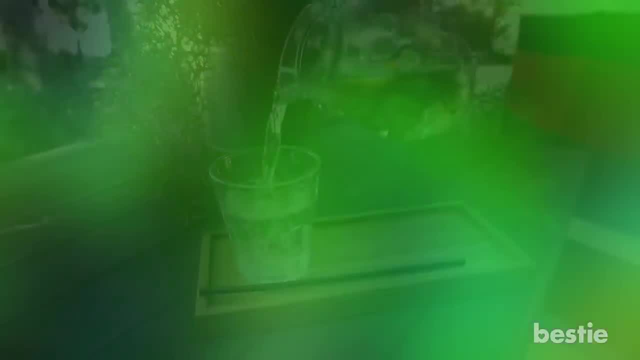 salads, rice dishes and, best of all, teas. You can also add fresh leaves to your smoothies, juices and drinking water. Want to keep learning about herbs like mint? Watch Seven Herbs and Spices With the Most Powerful Health Benefits, Or 14 Teas to Lower. 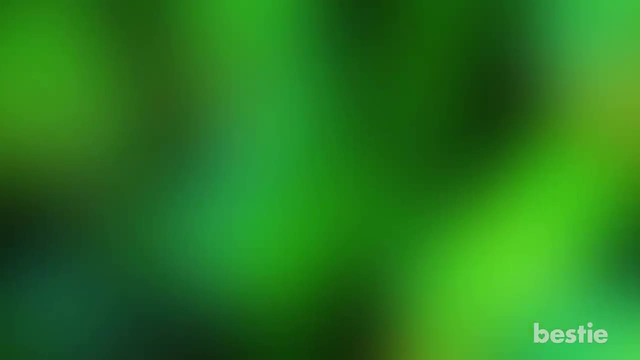 cholesterol, high blood pressure and clean clogged arteries. Click one, or why not both, and keep the conversation going, shall we? Are you adding mint to your daily diet and routines? Let us know in the comments below.